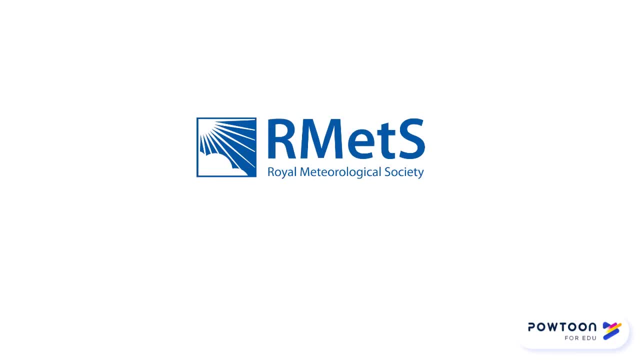 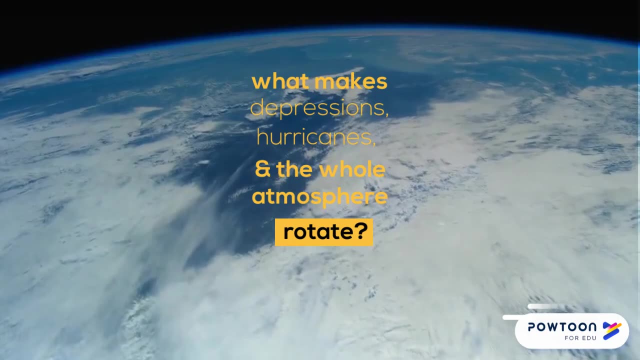 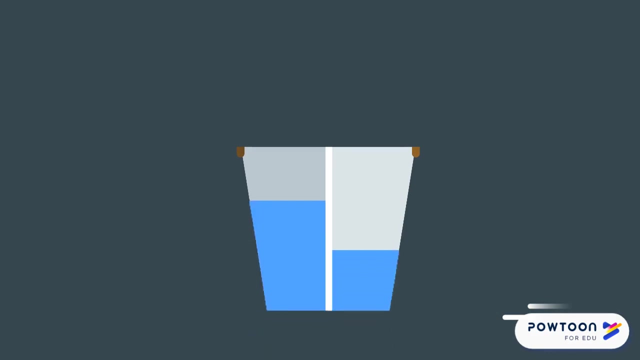 What makes depressions, hurricanes and even the whole atmosphere rotate? In fact, what makes air move at all? Imagine you have two containers of water, one holding more than the other, and you take the barrier between them away. What happens? The water flows from where there is more. 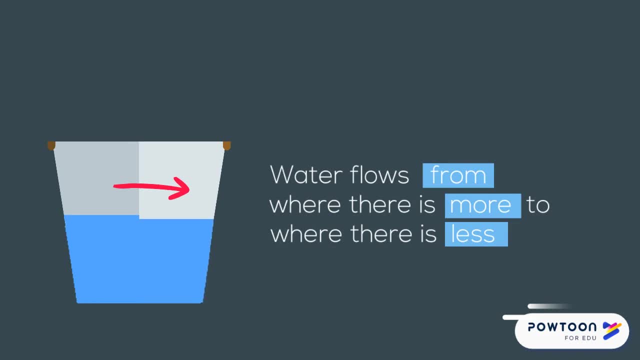 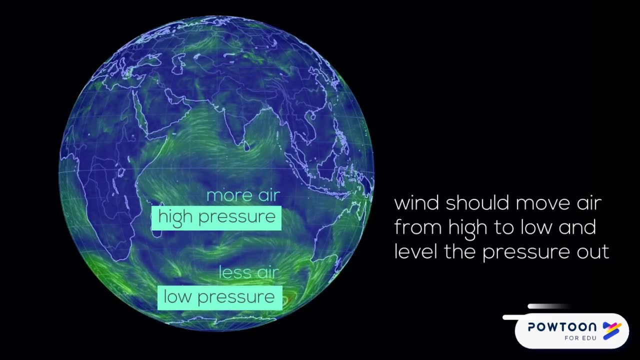 to where there is less and the water levels out. So in the atmosphere, if there is more air in one place- high pressure- and less elsewhere- low pressure- the wind should move air from high to low and level the pressure out. But this doesn't happen. The wind blows along the pressure contours. 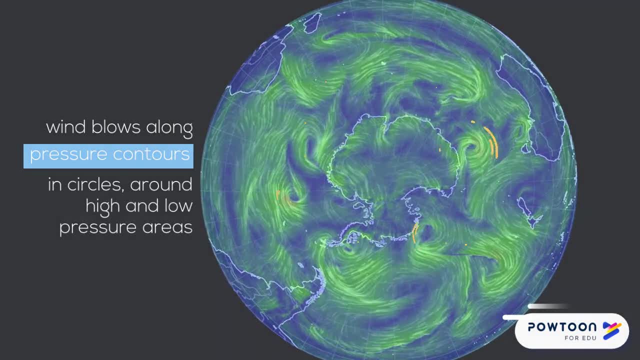 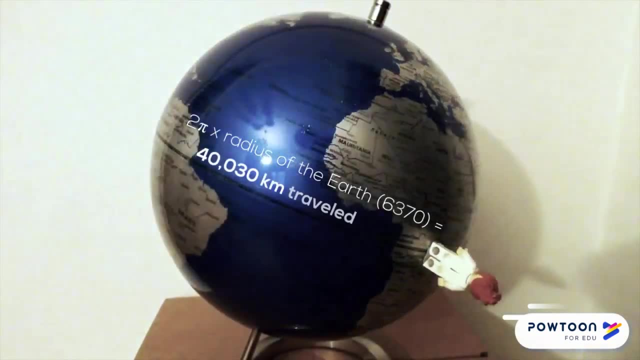 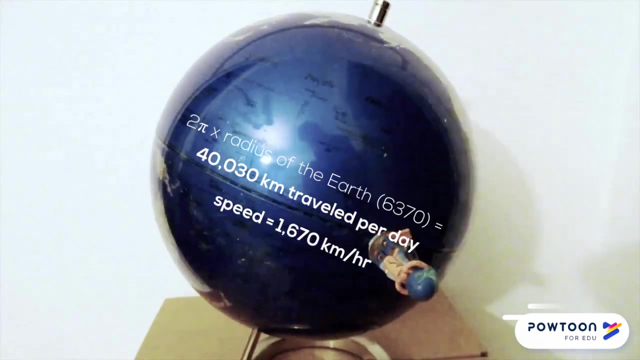 in circles around high and low pressure areas. Why? Imagine you are standing at the equator. In the course of a day, you travel about 40,000 kilometers a speed of about 1,670 kilometers per hour. You don't notice it because the air around you is also traveling. 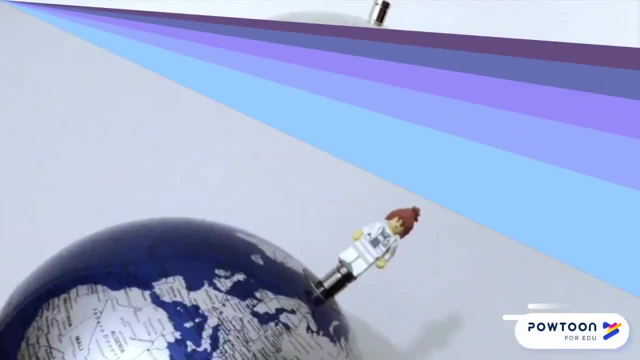 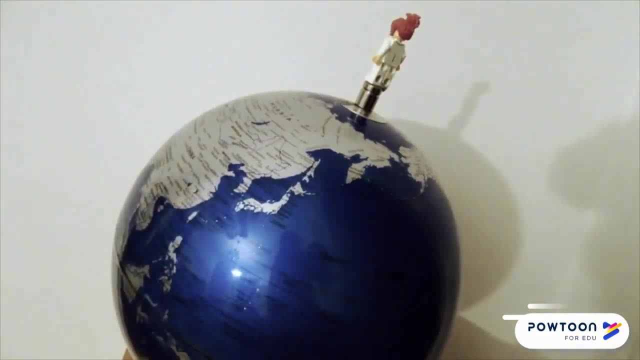 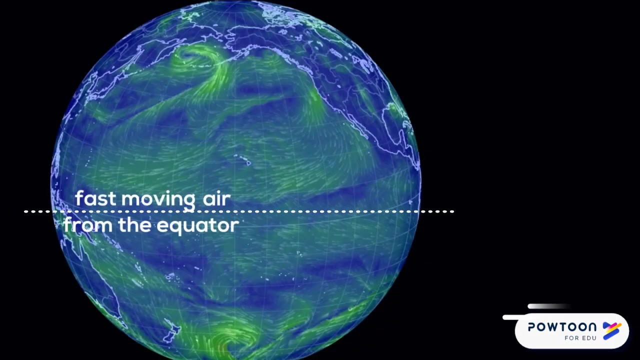 at the same speed, So there's no wind. On the other hand, at a pole, over the course of a day you would stay in the same spot, but just turn 360 degrees. You and the air around you aren't traveling at any speed at all. So if fast-moving air from the equator is pulled towards the poles, 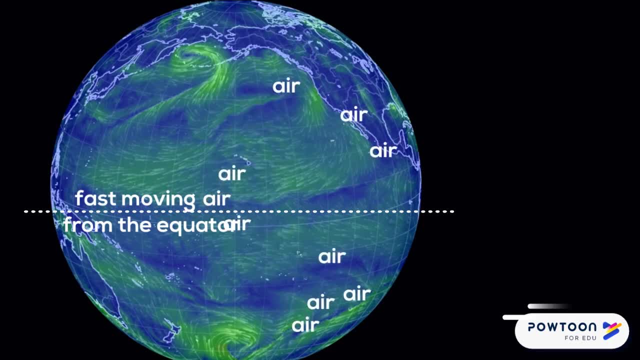 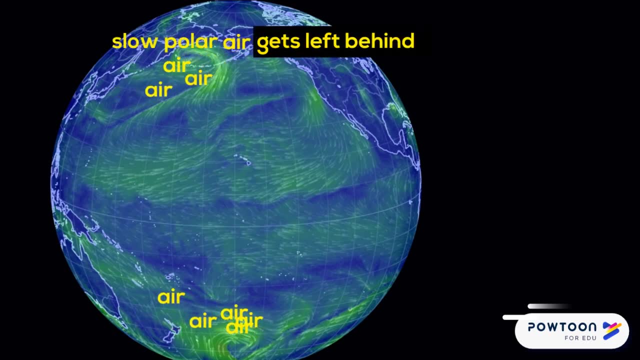 it is traveling faster than the ground underneath it and it overtakes it. On the other hand, slow polar air gets left behind if it's pulled towards the tropics. So any air trying to move south or north can't travel in a straight line but ends up moving progressively. 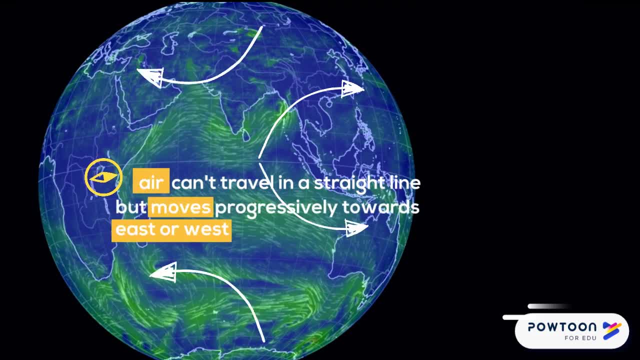 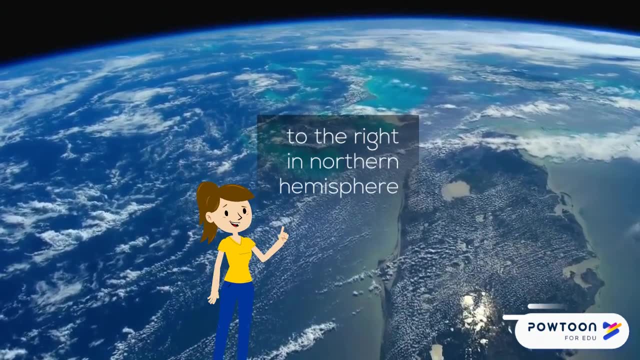 towards the east or west. More generally, the Coriolis effect tells us that moving objects on the surface of the Earth are always deflected to the right in the Northern Hemisphere and to the left in the Southern Hemisphere. It's all due to having to consider what the Earth's rotation. 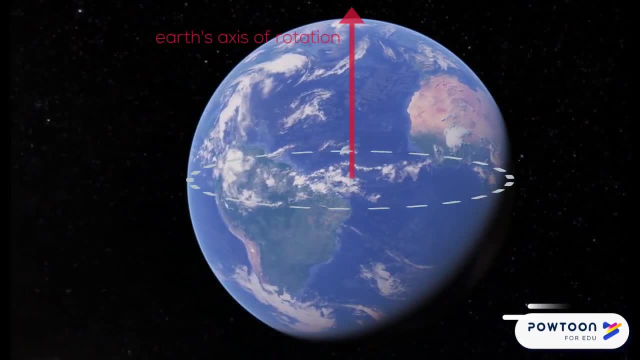 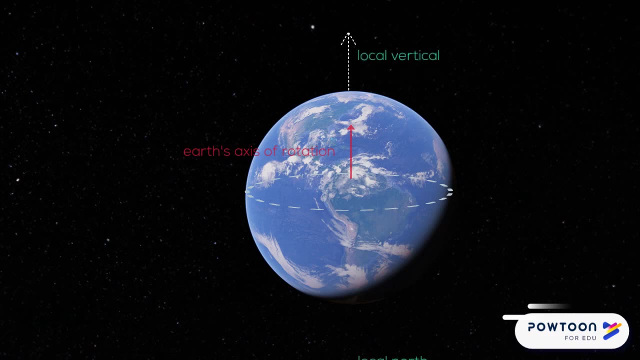 looks like to someone on the ground. To understand the local effect of the Earth's rotation you have to split it into components around the local vertical and the local north. To people standing in different places, north and vertical could mean different directions. At the equator, the component of the Earth's